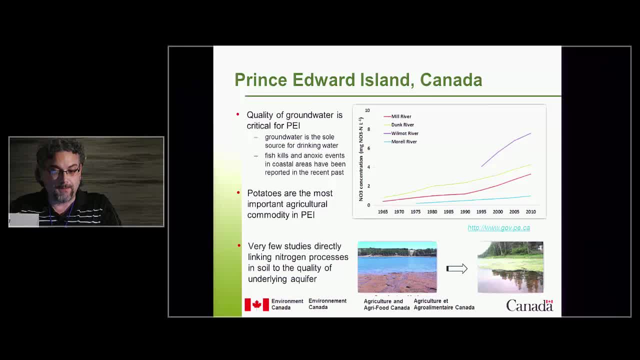 Agriculture plays a significant role in local economy, with potatoes being the most important commodity. This graph here Shows nitrate concentrations in several streams in Prince Edward Island between 1960s and 2010.. And we can see that concentrations increased two or even three times compared to the pre-intensive ag practices. 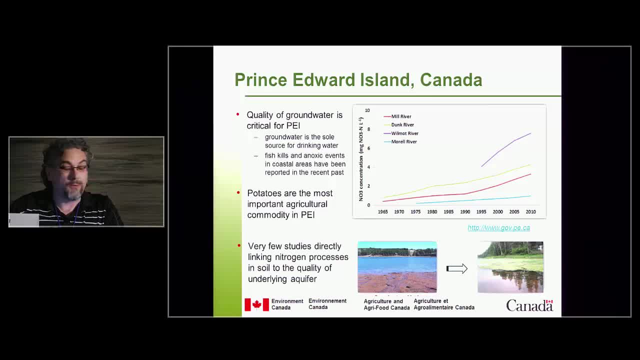 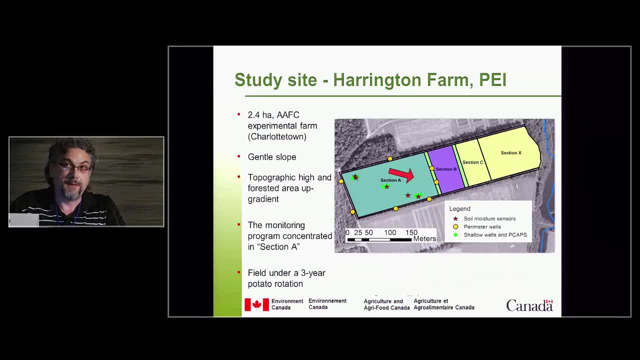 which have been linked to a decline in groundwater quality. The study site is at the Is at an AFC Agriculture and Agri-Food Canada experimental farm close to very close to the provincial capital, Charlottetown, And the field site is set in a healy landscape with a topographic height just above. 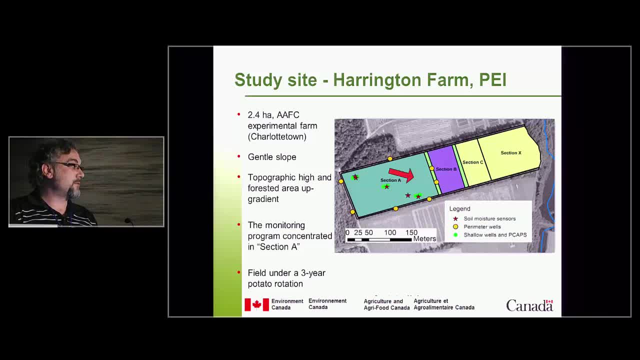 just up gradient of the field here where there's also a forested area. So monitoring took place mainly in this section of the field with seven perimeter wells that are in the middle of the field. These are intersecting or capturing the top up to six meters of the regional aquifer. 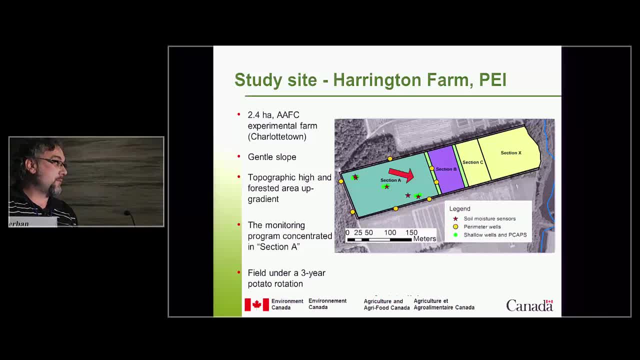 For this presentation or work. these three wells that are up gradient were labeled as low nitrogen wells as they always had concentrations much lower than this group here of four wells which are labeled as high nitrogen wells. In the field there's three nests of three piezometers as well here, following the groundwater flow direction. 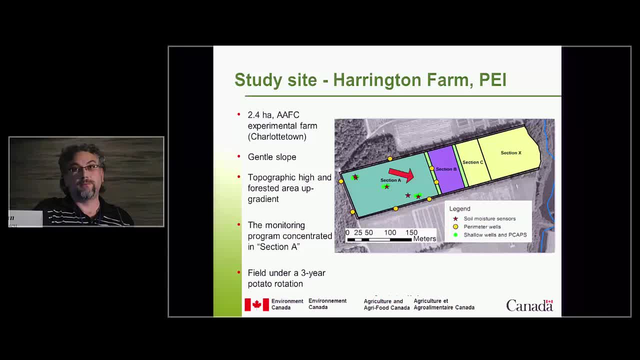 And in each nest we have three wells- shallow, intermediate and deep- And they capture, they intersect the top. So they were drilling in such a way that they would capture the top two meters of the aquifer at any point during the year. 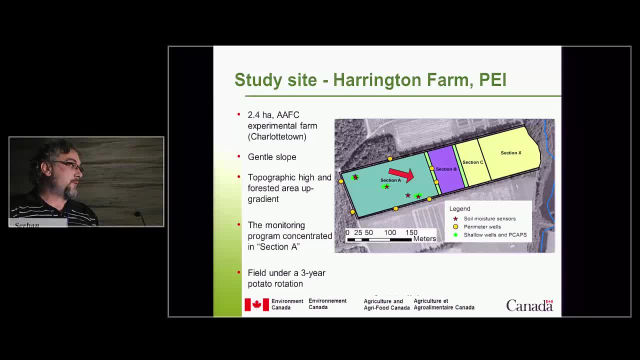 There's at each nest. there's also. we have four P-caps, passive capillary samplers or weak samplers, installed just at the bottom of the root zone for obtaining cumulative samples of leachate from the crop, And with the red stars several locations are monitored continuously for soil moisture temperature. 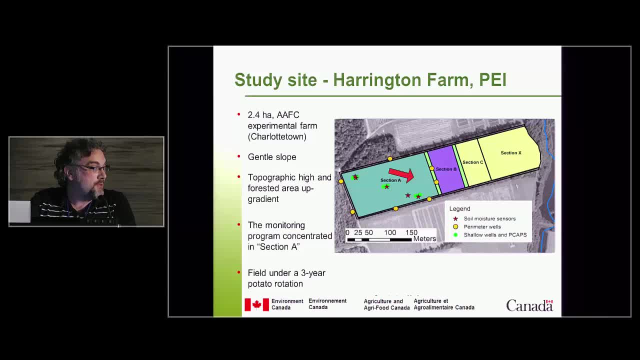 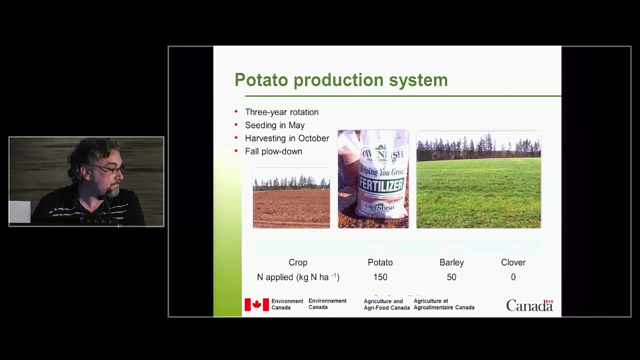 and electrical conductivity. At each location we have up to four depths monitored between five, ranging between five and 80 centimeters deep. This field is under a three-year rotation. potato rotation, which is a potato barley clover rotation, with the potatoes receiving about 150 kilograms of nitrogen per year. 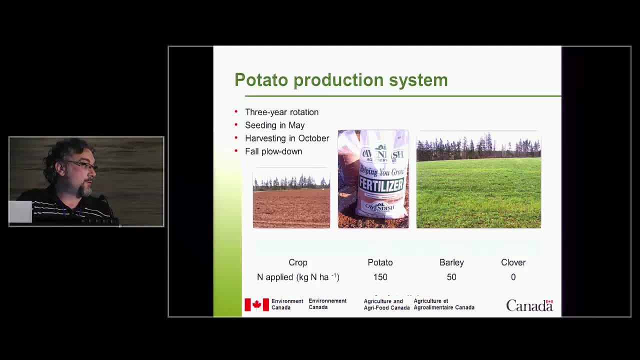 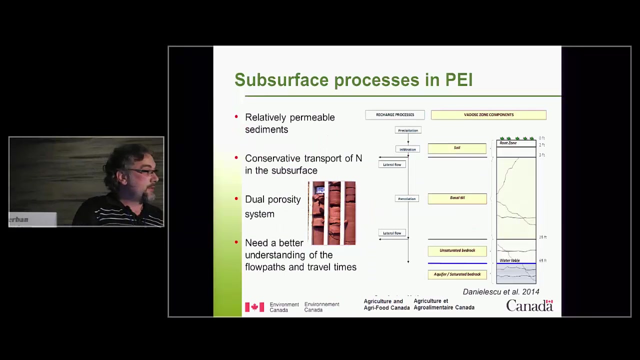 Barley, 50 kilograms- And no fertilizer. No fertilizer applied to the clover crop. Seeding typically takes place in May, depending on the weather, with harvesting usually in October. The soil at the site is about. the soil layer is about three meters deep, with three horizons. 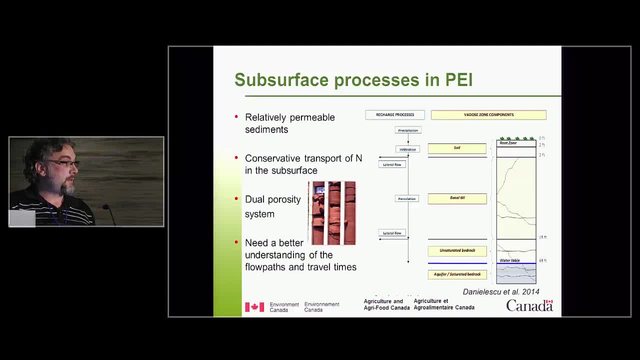 Root zone extends down to 60 centimeter And the soil layer is underlain by glacial till down to about eight meters. Below that, we have the sandstone bedrock, with the water table at about 20 meters depth, And both the till and the bedrock are fractured. 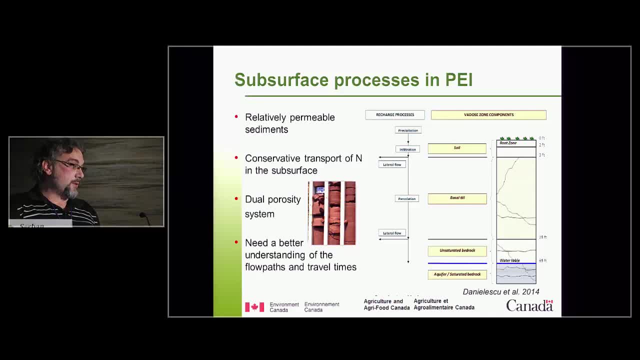 And I included here a core, a picture of a core, just for showing The typical fractures that we see. Both the all the sediments, soil, till and bedrock are permeable And typically the nitrogen transport is considered to be conservative. 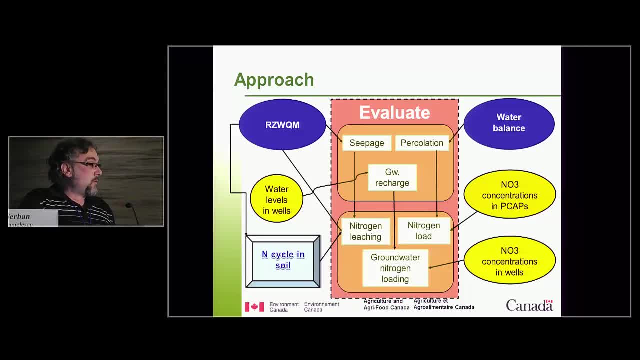 So here is the approach. So in the first step, a model was developed. The model was developed under, with the root zone water quality model, a USDA model Able to simulate the flow nitrogen cycling in soil and plant growth. So as a result of that, we have obtained estimates of seepage water leaving the soil profile through the bottom boundary. 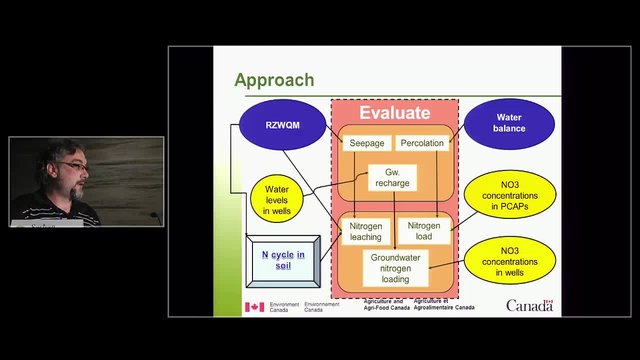 As well as detailed budget of nitrogen cycle, Of nitrogen processes in the soil, One of them being nitrogen leaching, which will be discussed here. Through a separate effort, a water balance was calculated Or a water budget was calculated which provided estimates of percolation. 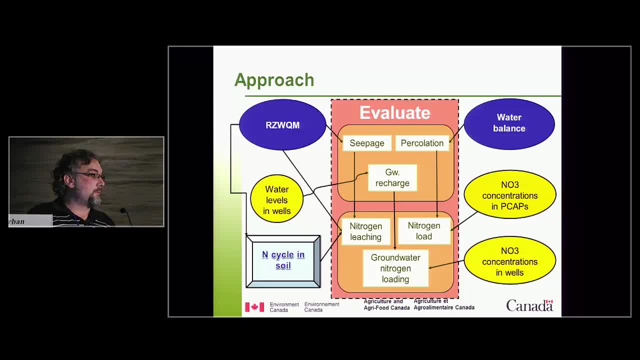 Again, water leaving through the bottom of the soil profile. This percolation in conjunction was used together with the nitrate concentrations in the passive capillary samplers To obtain nitrogen loading that would be available for moving towards groundwater. And yet through a different, another effort. 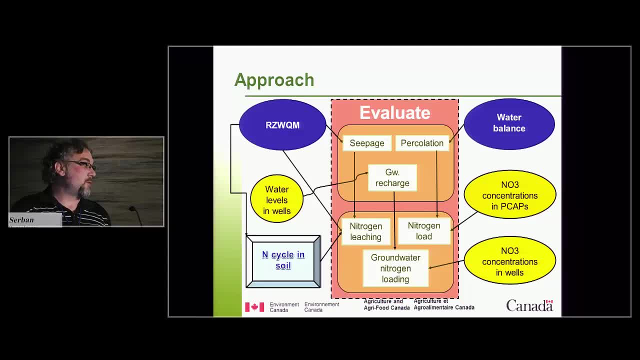 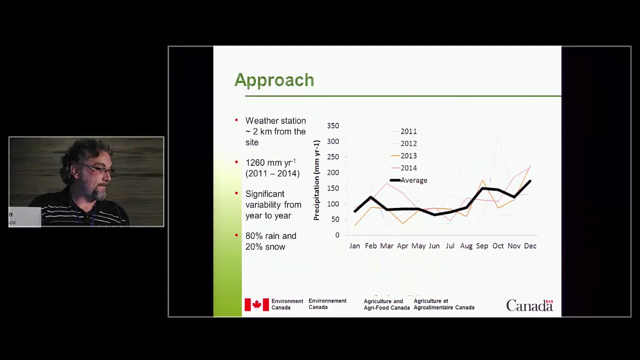 Groundwater recharge was estimated using water levels, Changes in water levels In the perimeter wells, And that was used together with the nitrate concentrations measured in the wells To obtain the groundwater nitrogen loading. This is just showing variability of precipitation Over the four years of the study. 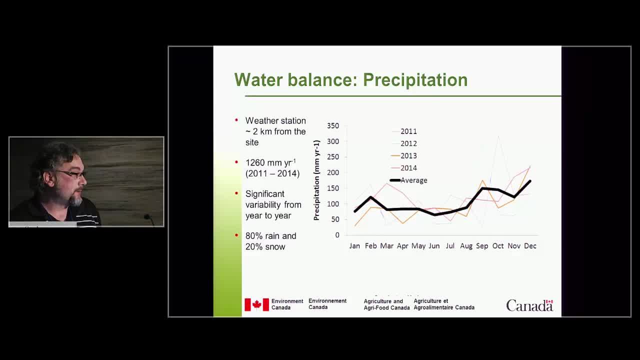 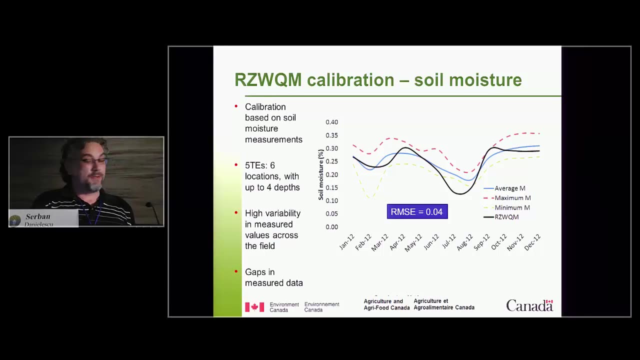 Significant variability And on average we're looking at about 13%- 1,500 millimeters per year. 20% of that falls as no. So the calibration target was the model was calibrated such as to minimize the differences Between the calculated soil moisture and the measured soil moisture. 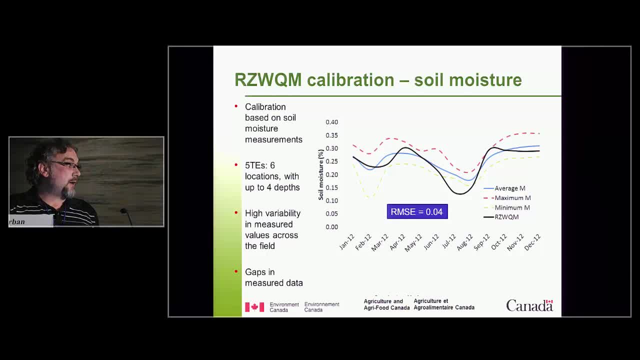 So black line here shows the model output, Whereas the blue line shows the average of measured soil moisture. This is for 30 centimeter depth And we can see that generally there's good agreement Between the two data sets. However, here during the summer months, 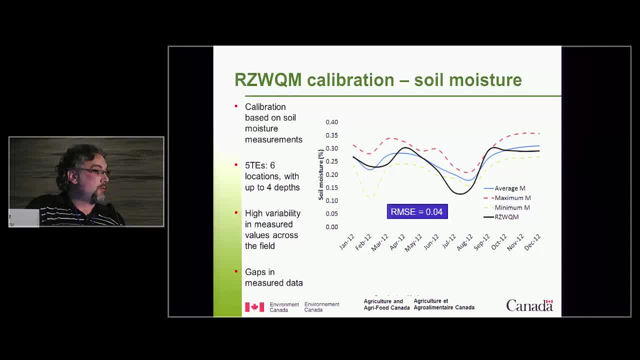 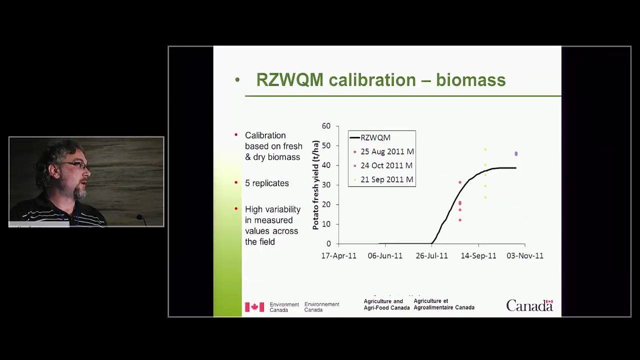 Roots on water quality might provide lower values compared to the measured data. We can also see this Sometimes. we have significant Variability in measured data, Which makes the calibration challenging Or maybe easier actually. So this is another. Calibration was done also for plant. 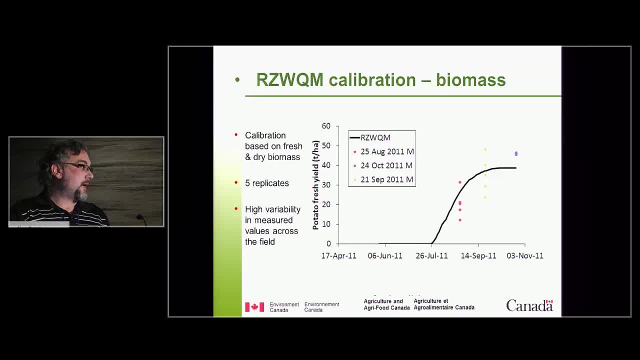 For the plant growth routine of the model And this is a graph showing the fresh yield for potatoes. And again we see the model. The output from the model Typically or usually falls within the measured values, But again we see high variability in measured values for fresh yield. 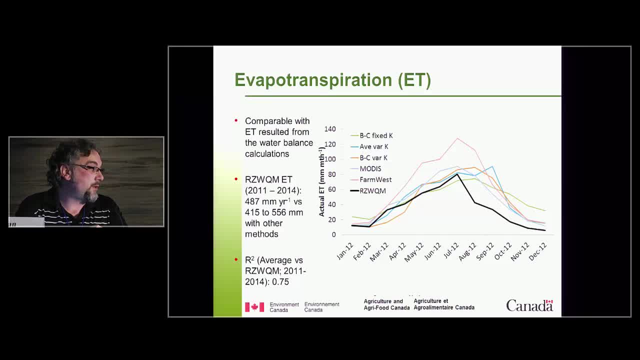 Evapotranspiration. Here is a comparison between the roots on water quality model Estimates And a number of other methods. Again, overall, good agreement in terms of annual amounts We see And also dynamics throughout the year. However, we see that for this particular year, 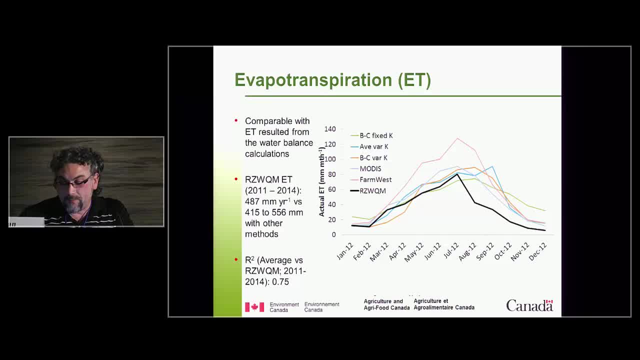 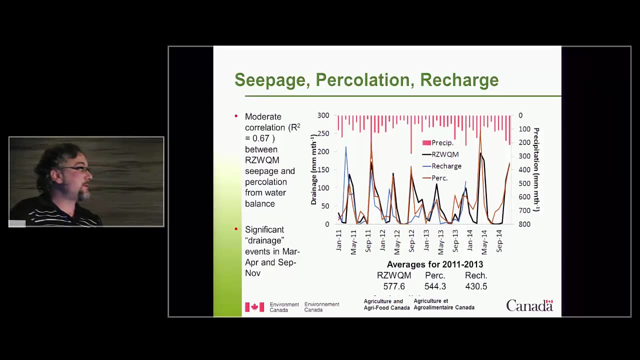 Roots on water quality model has Somewhat lower values for evapotranspiration When compared to the other methods. Here is a comparison between: seepage Obtained with roots on water quality model. Percolation Based on the water budget calculations. 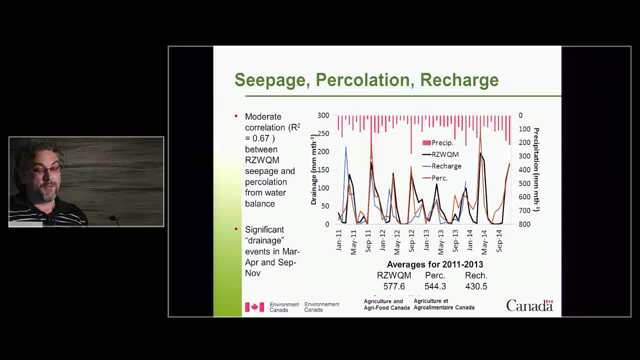 And recharge obtained from changes in water levels. So we see that generally, Typically, the peaks are in mid spring and mid fall. In mid spring, that recharge event is triggered by the snow melt. There is significant accumulation of snow over the winter. 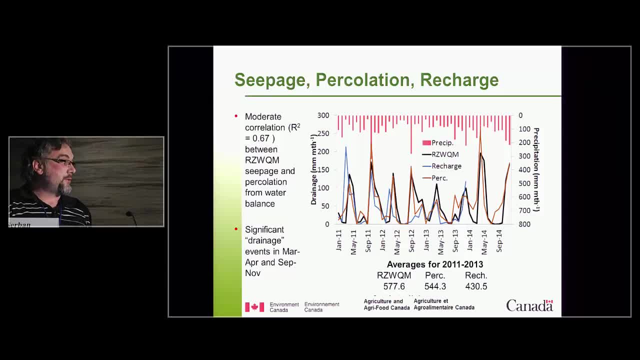 Whereas the one in the fall is generally triggered by increased amount of precipitation. Occasionally, we see a shift in peaks between the recharge Calculated using the water levels in wells And the peaks obtained through the other two methods. This could be Maybe. 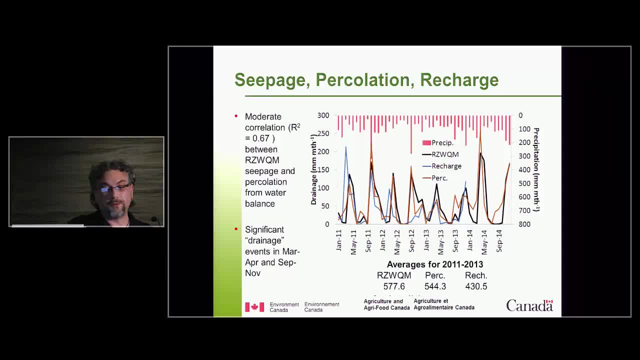 A result of Recharge Taking place Occurring earlier in the regional aquifer. Other than that, The Overall the recharge is, It's lower Than Than the annual estimates for For With the other obtained with the other two methods. 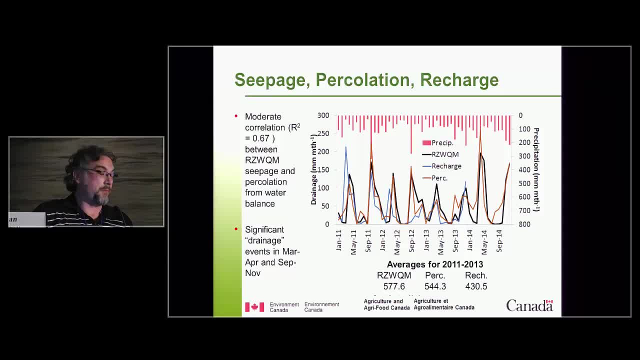 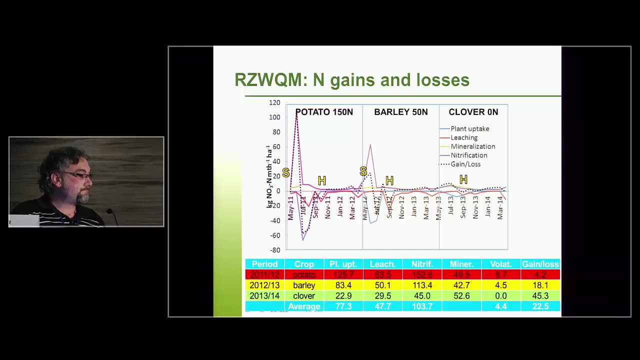 And that could be Due to a change in storage or Potentially, Maybe Potentially Lateral flow. Here is the Nitrogen budget. resulted The output from the model with respect to nitrogen budget? So above the X-axis. 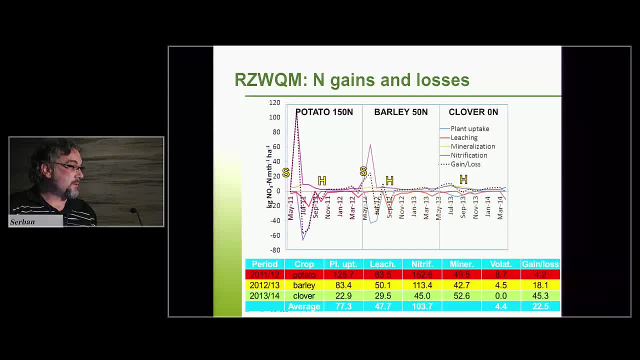 We have the gains And here we have the losses. So, in terms of gains, Nitrification and mineralizations are the largest ones. Nitrification, So Conversion of Ammonium to nitrate, Has huge peaks Here, immediately after seeding with S. 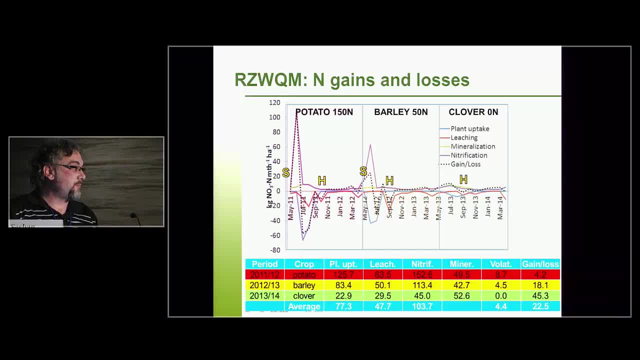 Not noted with S. So we see those, These kind of peaks for both the potato phase As well as from For the barley phase, That there's no peak for clover when there was no Fertilizer applied Losses. 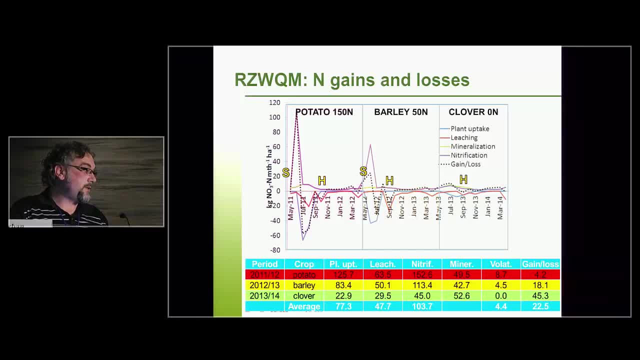 Plant uptake and leach Leaching are the most significant ones, With plant uptake Picking up during the summer And leaching Generally following The recharge events, With an exception here, Where Where there was a buildup of nitrogen in the soil. 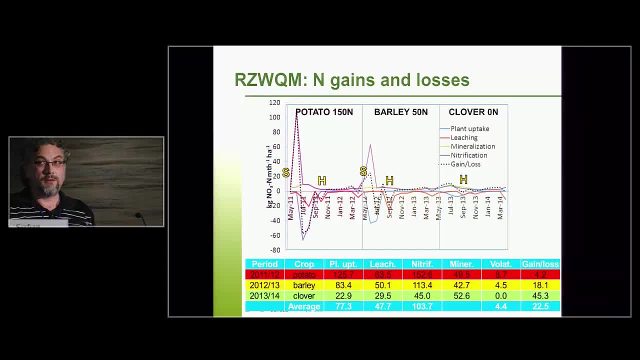 And it Took advantage Sort of Of the first Month With Nitrogen In the soil And It Took advantage Sort of Of the first Month With Nitrogen In the soil And 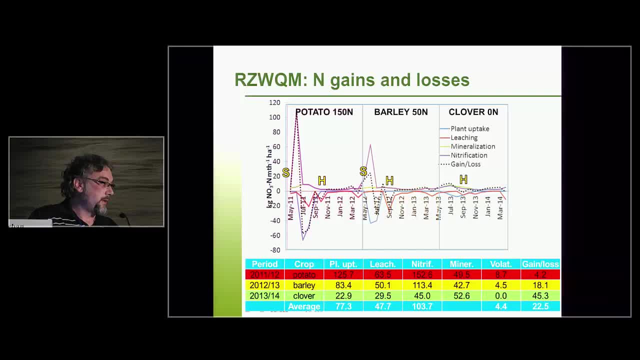 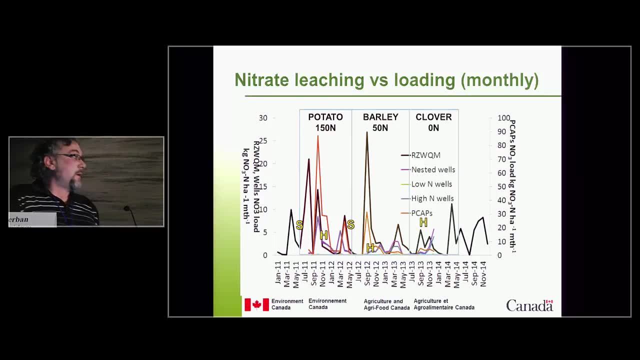 A month With With Some Recharge Available In order to be Flushed out. So Here Is The Comparison For Nitrogen Loading Or Leaching With Root Zone. 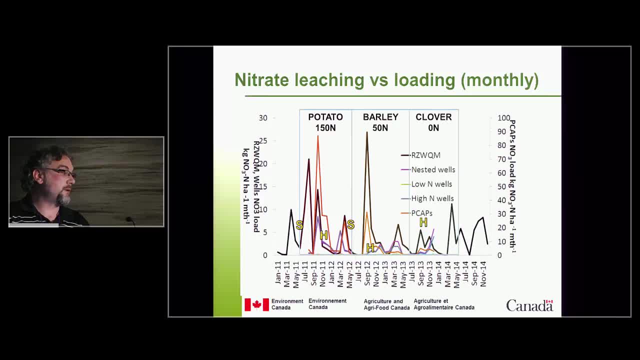 Water Quality. Nitrogen Leaching. Nitrogen Leaching Obtained With Root Here On The Secondary Axis, Just Because There Were The Estimates Were So Much. 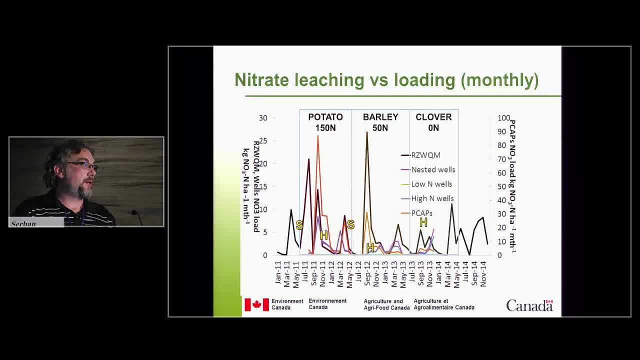 Higher Than The Estimate, The Estimates Obtained With The Other Methods, And There Have Been Across The Field, And So These Data Should Be Used. 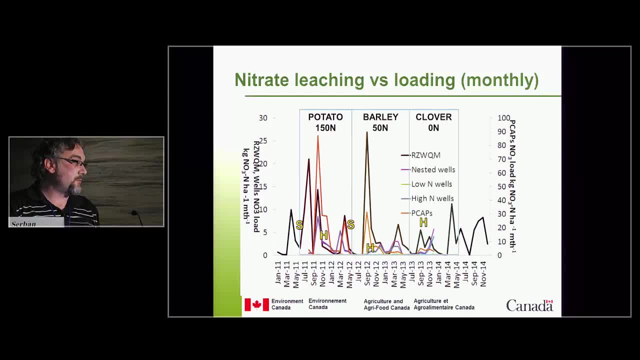 With Caution. The Other Thing Is We Don't Have A Complete Data Set For Concentration, So We're Missing A Occasionally. We Might See That. 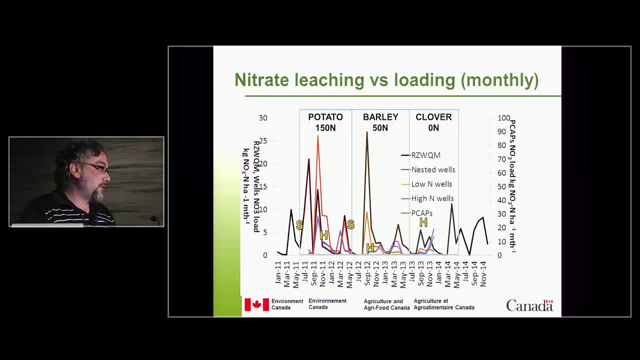 Shift That Was Seen For The Drainage Or For The, For The Previous Slide Showing Just The Flows And What The Other Thing We Are. 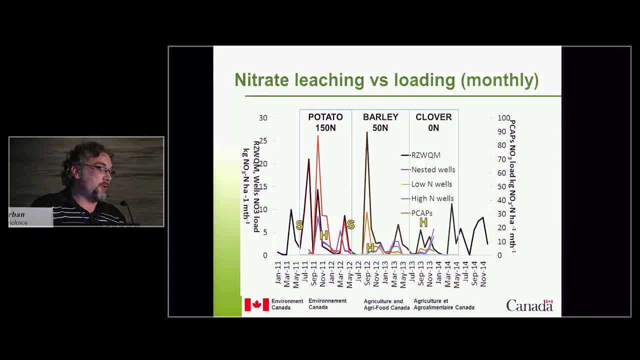 Thinking That, If We're Thinking About The Dilution Of Water Coming From The Field, With Water From The Regional Aquifer That Is Lower In, 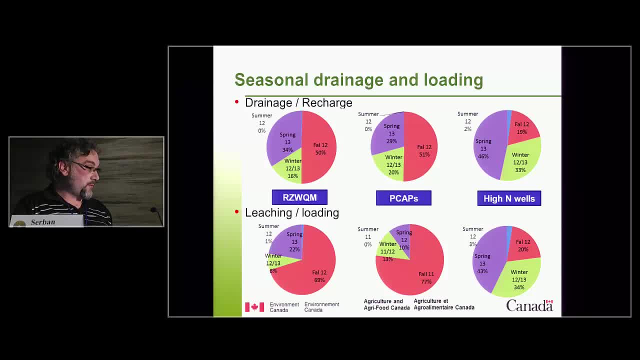 In Has Lower Concentration Of Plants. There's Generally Good Agreement With With The Fall Dominating Both The Drainage And The Leaching Slash Loading. 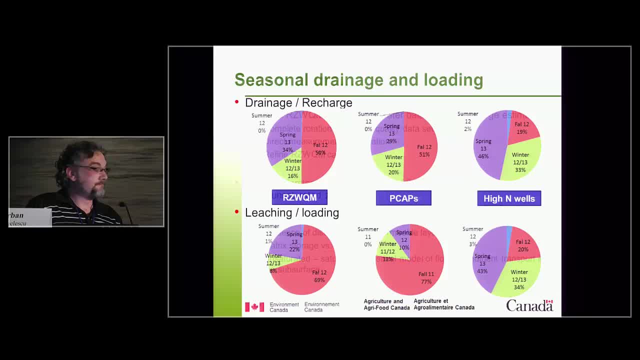 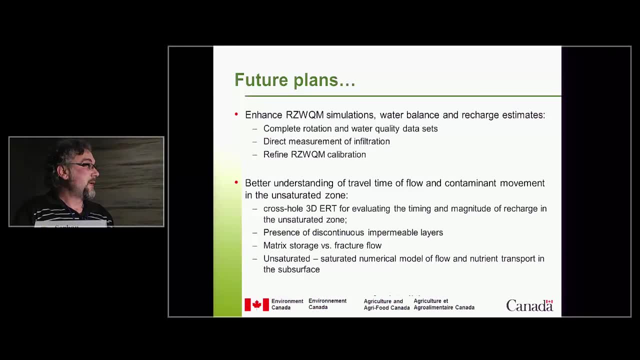 Processes And With The High End Wells, Again We See A Different Way To Enhance These Calculations And These Calculations Would Benefit For From. 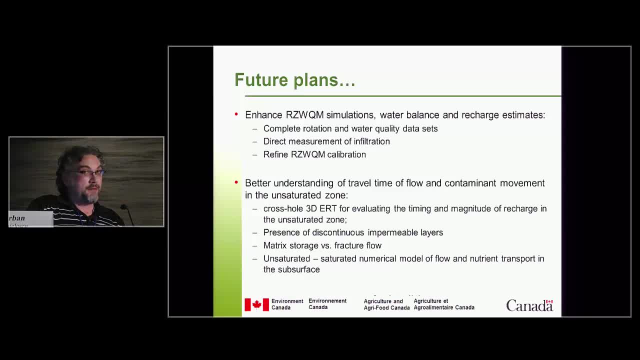 Having A Complete Data Set For Water Quality, A Better Method For Measurement Of Infiltration And I'm Really A Larger Effort Where The Aim 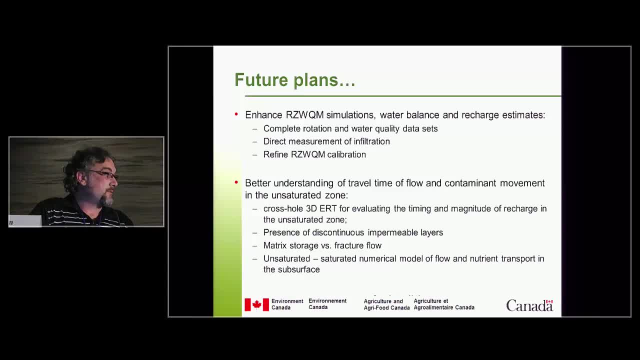 Is To Better Understand Travel Time Of Flow And Contaminants In The Unsaturated And Actually Saturated Zones. So There's Other Pieces Of Work. 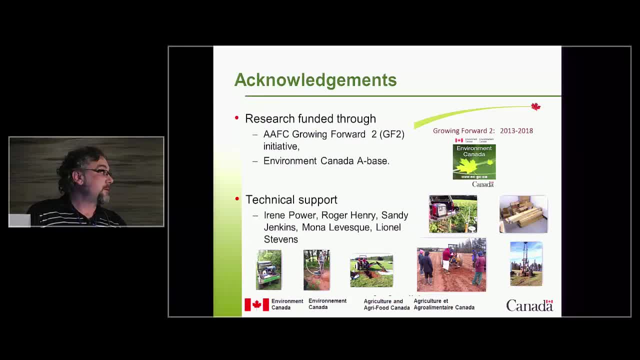 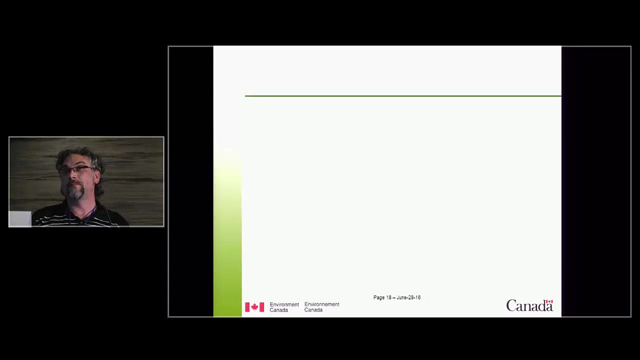 Taking. And This Is The Last Slide. Just I Would Just Like To Acknowledge The Funding Agencies And Technical Support Throughout The Program And With 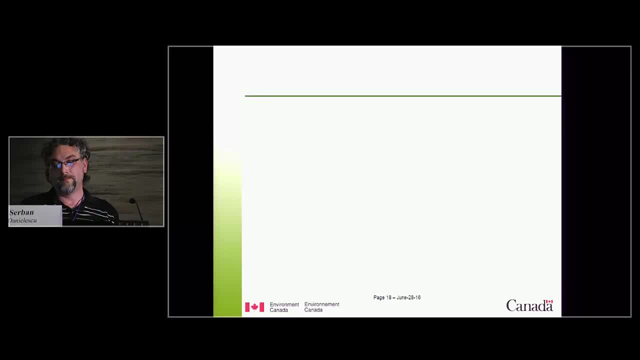 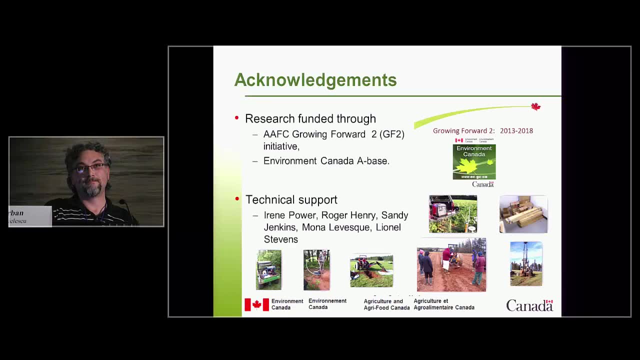 That, Thank You. Thank You. I Have A Few Questions, If I May The One. The First One Is About These Devices You Call The Pickups. 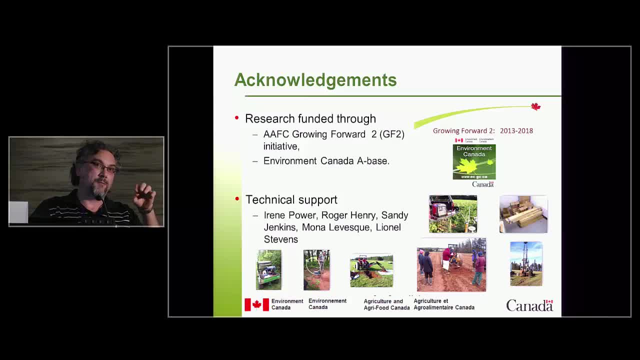 The Passing Capillarity Devices Are Those Type Of Infiltration. So You Are Able To Sample To. You Are Able To Obtain Cumulative Samples. 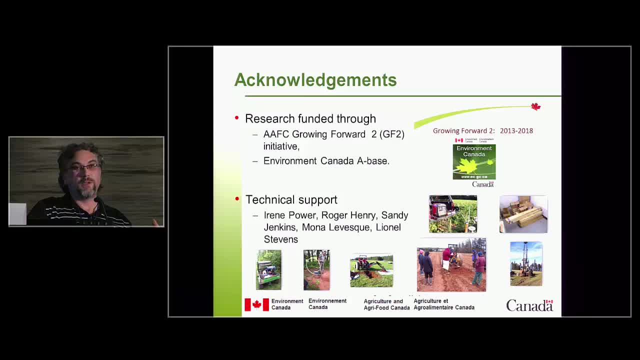 Sample. So In Theory You Are Able To Sample The Volume Of Infiltration Over Sample Campaign. Okay, And The Other One Was About The Water.